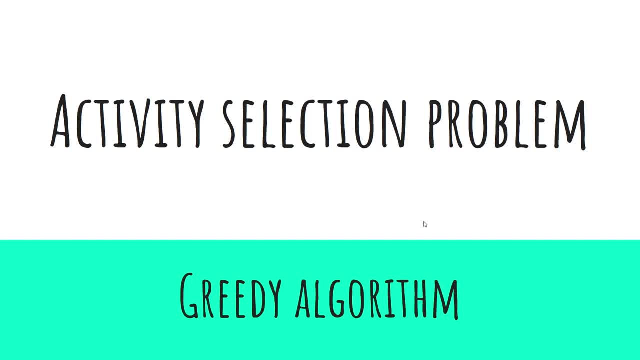 Hi friends, today we are going to look at activity selection problem using greedy algorithm. But before we proceed, if you haven't subscribed yet and you like what you see, do consider hitting the subscribe button. This encourages YouTube's algorithm in promoting more of our 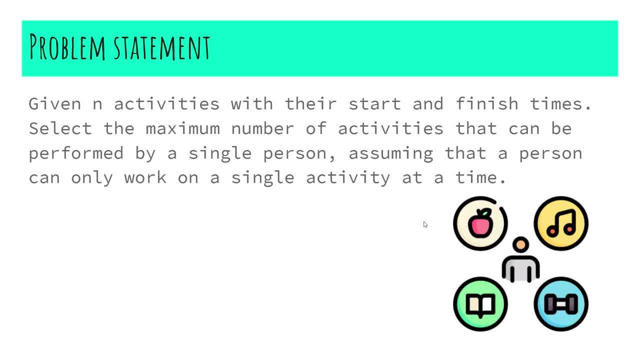 videos to more people out there. Let's look at the problem statement. Given n activities with their start and finish times, we need to select the maximum number of activities that can be performed by a single person, assuming that the person can only work on. 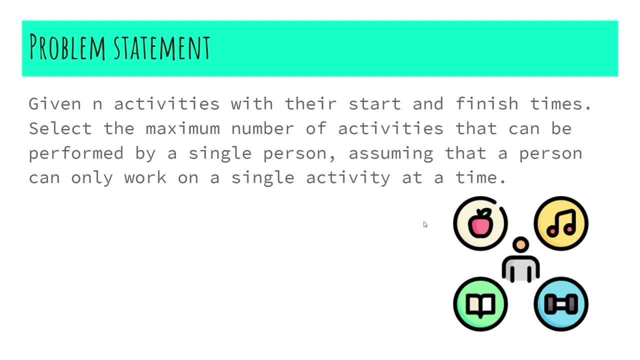 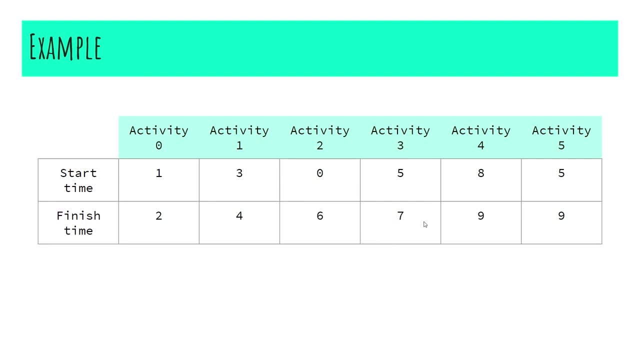 a single activity at a time. Let's look at an example. Let's say we have six activities, each with a different start and finish time. Now our objective is to pick maximum activities such that we can perform it without any time overlap. Let's assume we pick the first activity Since the finish time of the first activity. 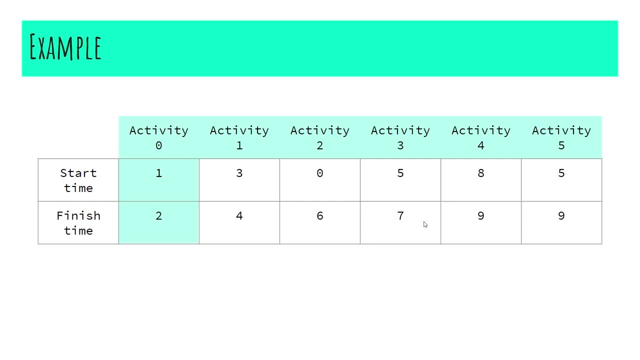 is 2, the second activity that we pick must start at a time with 2 or greater than 2.. Since activity 1 starts at time 3, we can perform both activity 0 and activity 1 without any time conflicts. Therefore, we tend to pick the activity 1 as well. Now, since the 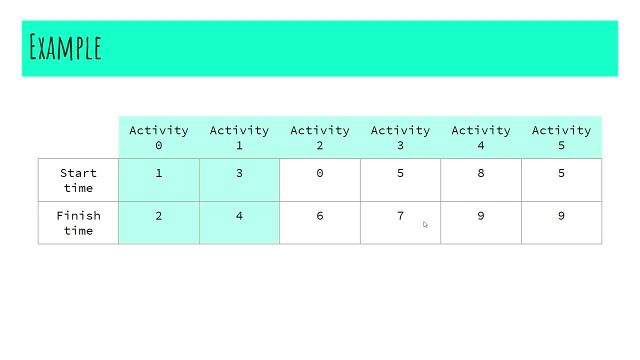 finish time of activity 1 is 4, we need to pick our next activity with the start time greater than or equal to 4.. Since the start time of activity 2 is not greater than or equal to 4, we jump to activity 3.. Since the start time of activity 3 is 5,, we can perform. 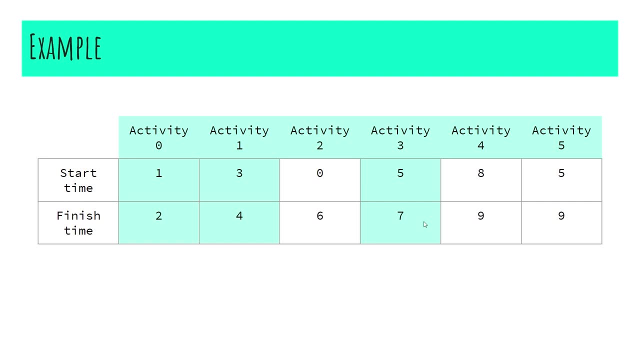 activity 3 without any time conflict. Before we proceed, the next activity that we pick must obviously start with the time 4.. Since activity 4 fulfils our constraint, we can pick activity 4 as well. Activity 5 cannot be picked since the start time of activity 5 is 5, but the last activity 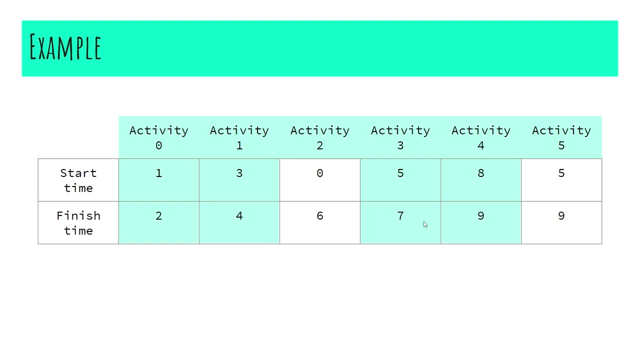 that we have picked, which is activity 4, ends at time 9.. Therefore, we cannot pick activity 5.. Therefore, at the end, we will be performing 4 activities, that is, activity 0,, activity 1, activity 3 and activity 4.. 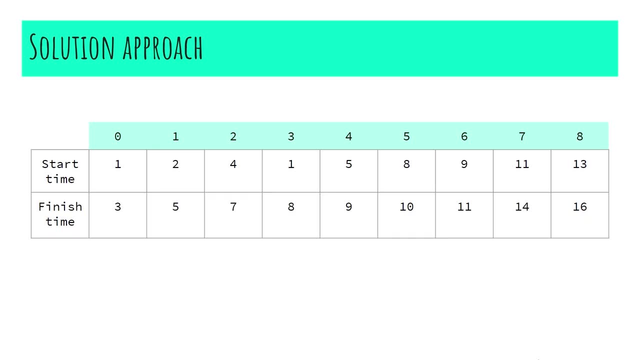 Let's look at the solution approach. Let's assume we are given an array of activities and each activity has a start time and a end time or a finish time. For this instance, I have taken an array with 9 instances of activities. We will begin with our iteration. 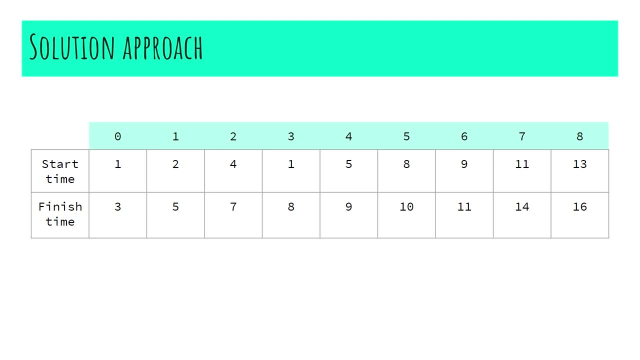 from the 0th position. At first we will pick activity 0 and then, as we iterate, we will compare the start time of the current activity with the finish time of the lastly picked or lastly selected activity, Since our lastly selected activity is activity 0 and the finish time is 3, but the start time 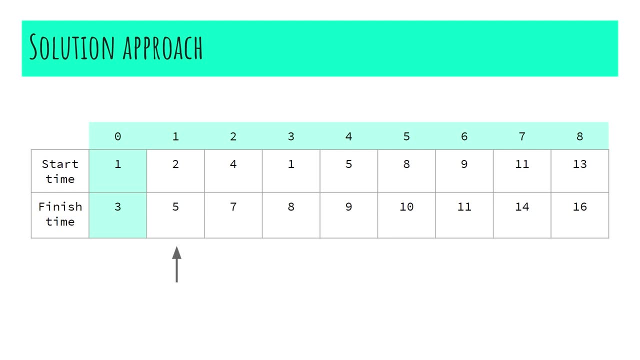 of activity 1 is not greater than or equal to 3.. Therefore, we will jump to activity 2.. Again, we are going to compare the start time of activity 2 with our lastly picked activity, which is activity 0. Since the finish time of activity 0 is 3, which is less than the start. 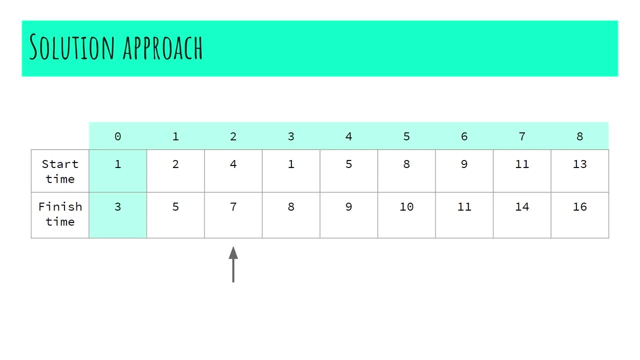 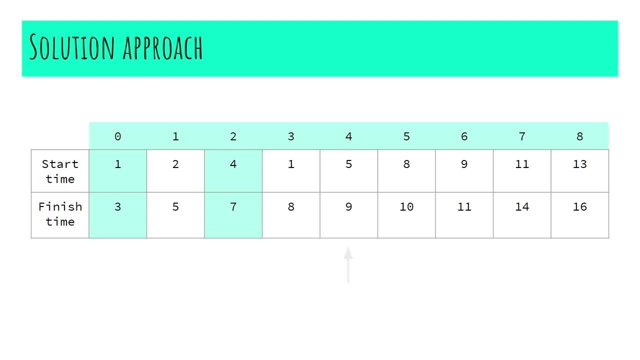 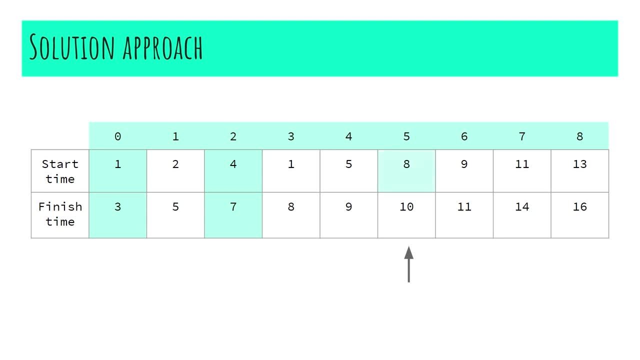 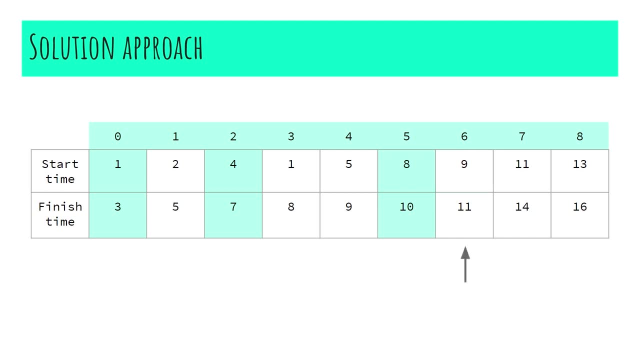 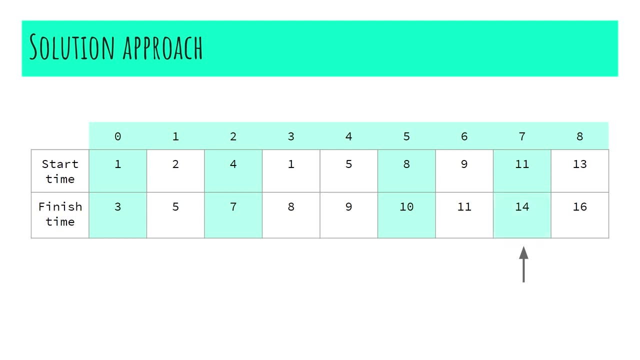 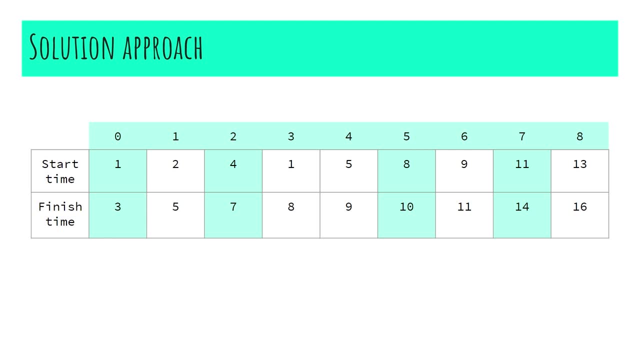 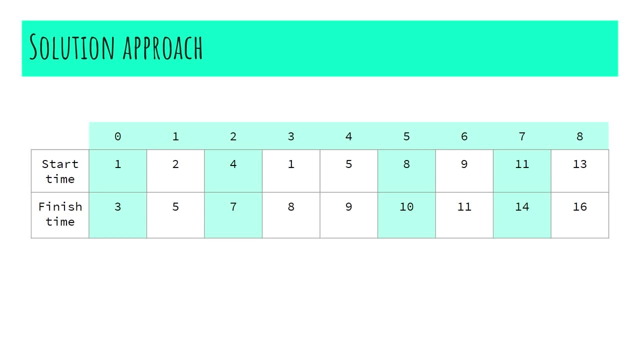 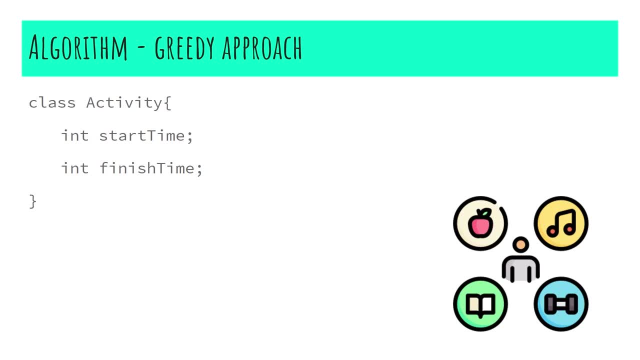 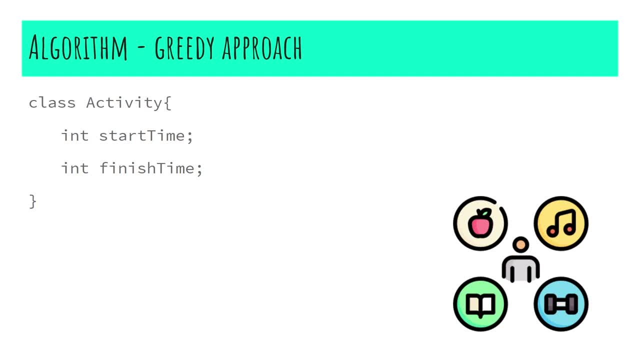 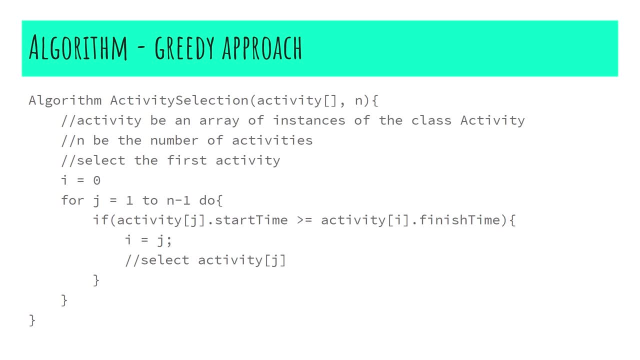 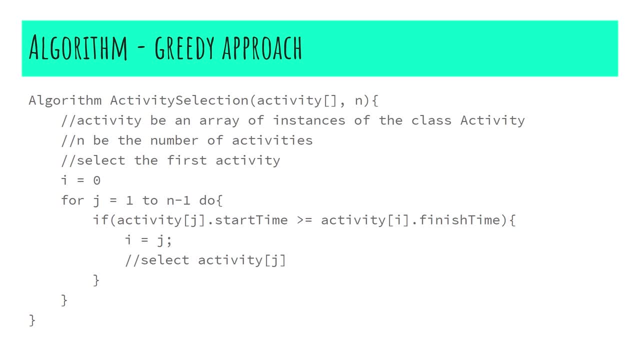 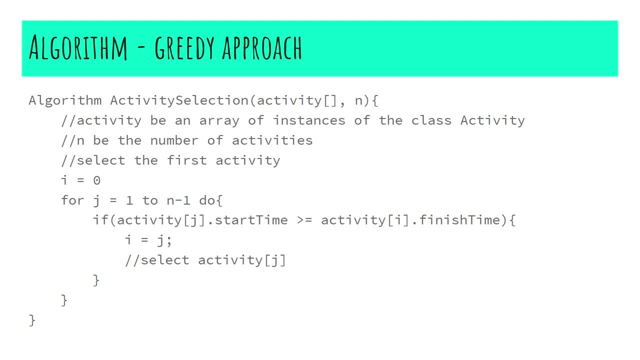 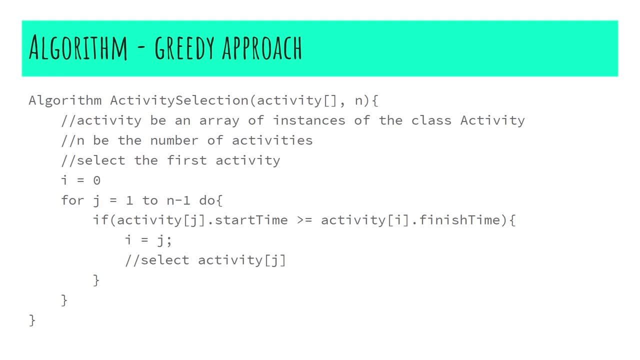 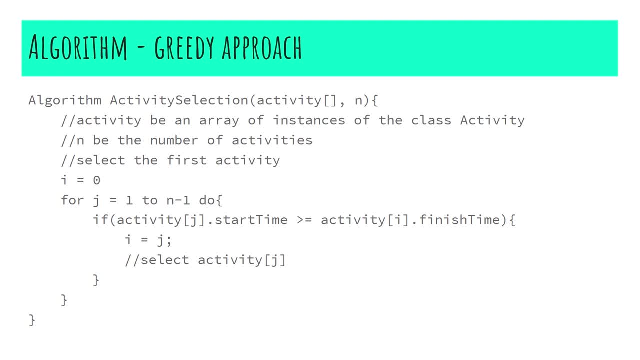 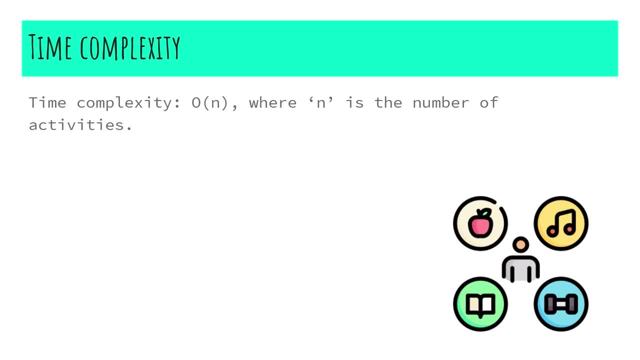